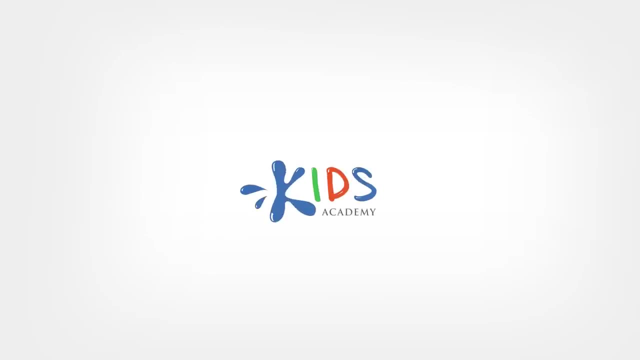 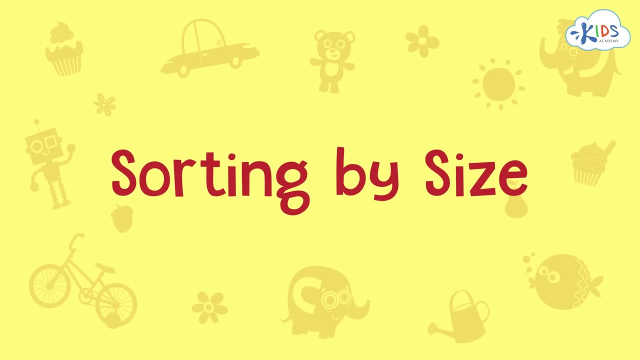 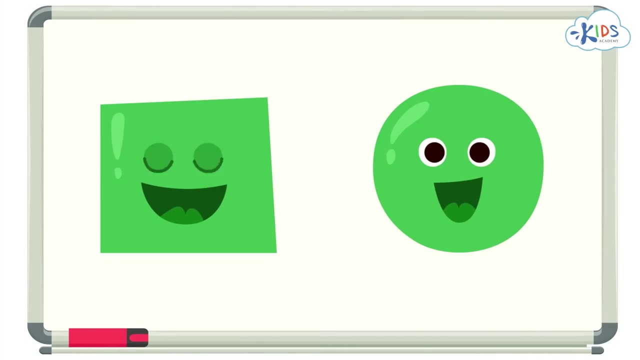 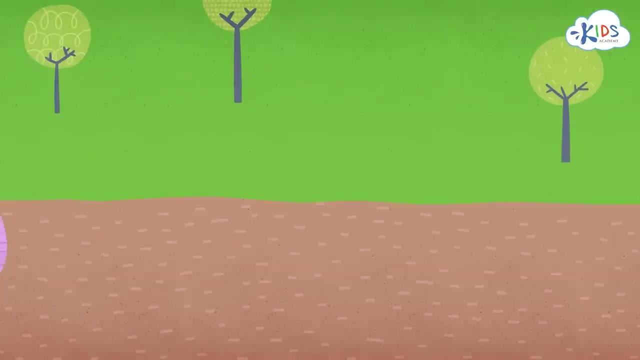 When we look at objects, we notice different things about them, like their color, their shape and their size. We can group objects together that are the same, like objects that have the same color or shape or size. Today, we're going to talk about sorting objects. 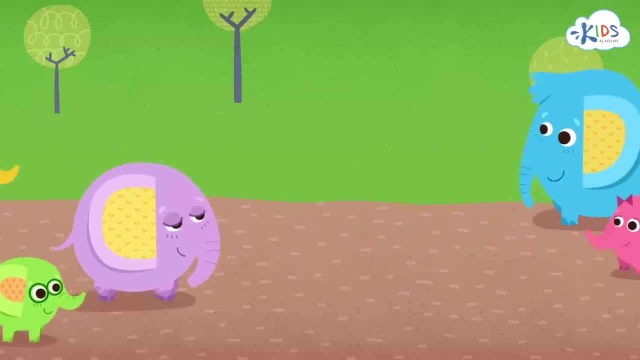 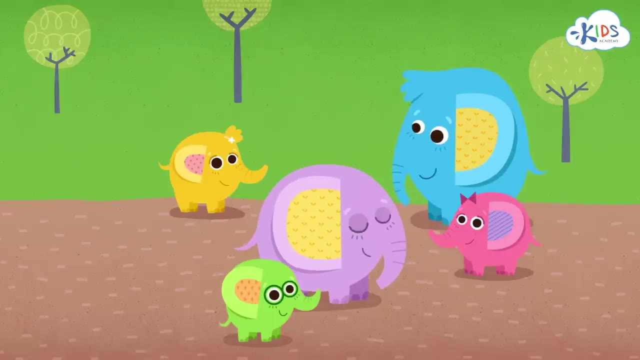 by size. Let's take a look at some animals. Look at all of these awesome elephants. There's Eddie and Billy. I also see three other elephants: Jackie, Jade and Jeffrey. I see big elephants and small elephants. One way we can sort or group these elephants is by size. Let's find. 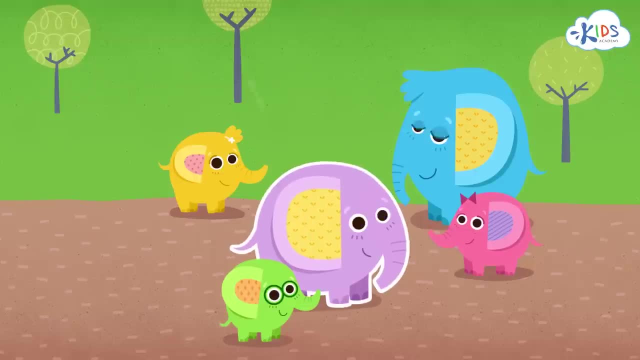 all of the small elephants. Eddie is a big elephant. He does not belong in the group with the small elephants. Billy is also a big elephant. He does not belong in the group with the other small elephants either. What about Jackie? Is she a big or a small elephant? 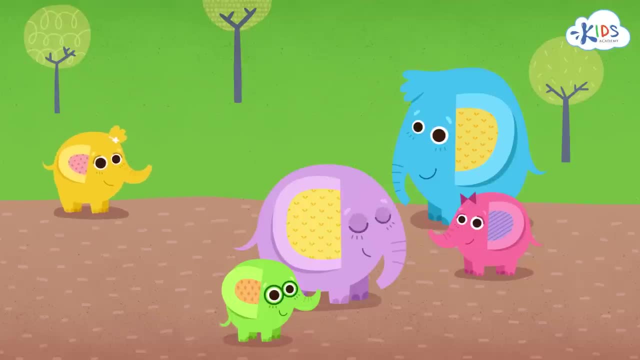 She's a small elephant. She must be a young elephant. She belongs in the group of small elephants. Jade is small too. She looks like Jackie. Maybe they're sisters. She belongs in the group of small elephants too. Whoa, check out Jeffrey, That's one cool elephant. 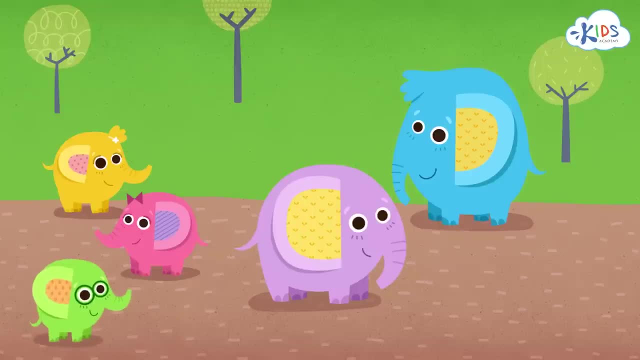 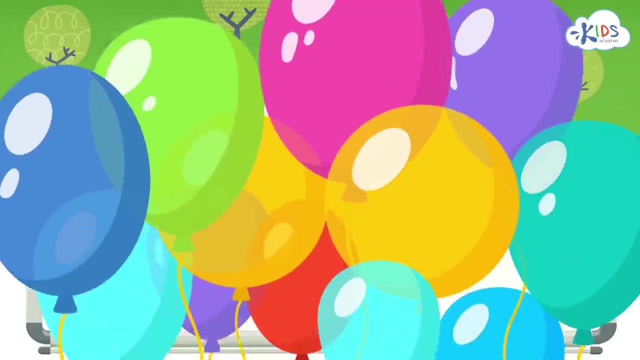 and he's small too, He also belongs in the group of small elephants. Are there any other small elephants? I don't see any Great job sorting these elephants by size. Let's try sorting one more group of objects by their size. Check out these cakes. I love cake. 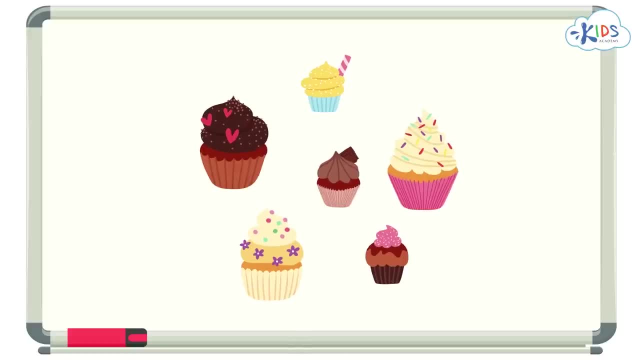 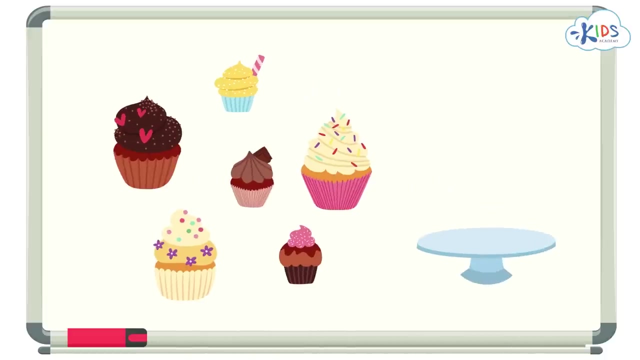 There's some chocolate cakes and vanilla cakes. Some cakes are big and some cakes are small. Yum, That's a lot of cakes and there's a few different ways we can sort them, But today we're going to sort them by size. Let's find all of the big cakes, because who doesn't?